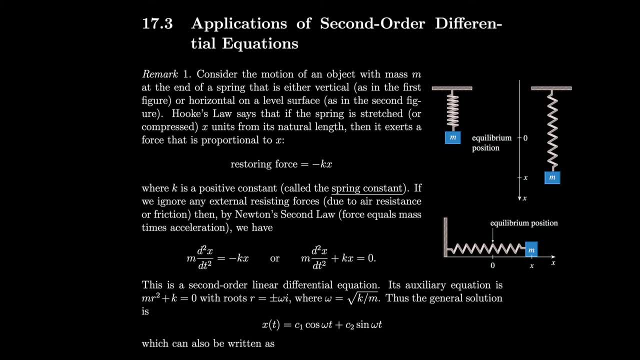 or friction, then by Newton's second law, force equals mass times acceleration. we have m times the second derivative of x with respect to t, equal to negative kx, which we can set equal to zero by just adding kx to both sides and we end up with a second-order linear differential equation. 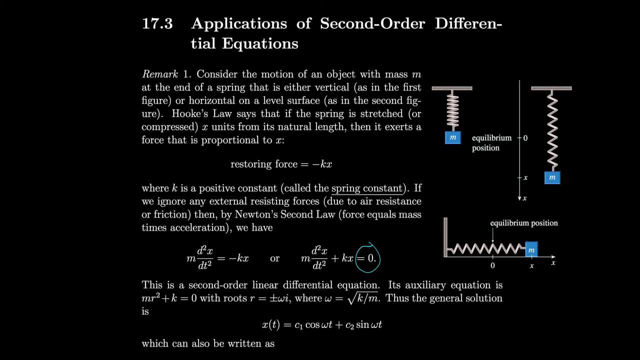 In fact it's even homogeneous because it equals zero. Its auxiliary equation is m times r, squared plus k equals zero, With roots plus or minus omega i, where omega is the square root of k over m. So you could just use the quadratic formula for that, And then our general solution must be: x of t equals c1 times. 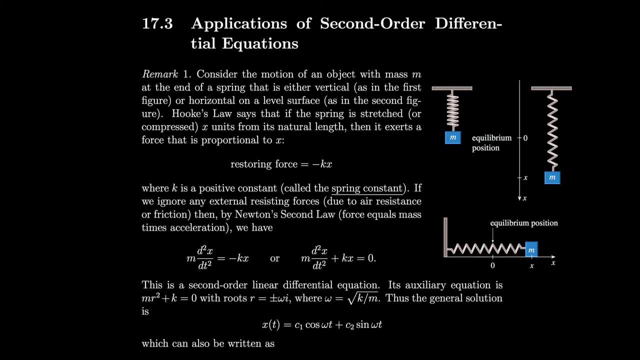 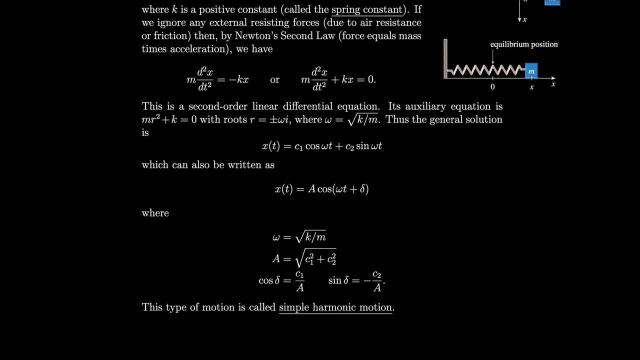 the cosine of omega t plus c2 times the sine of omega t. We can also write this, though, as x of t equals a times the cosine of omega t plus delta. where omega is the square root of k over m, a is equal to the square root of c1 squared plus c2 squared. 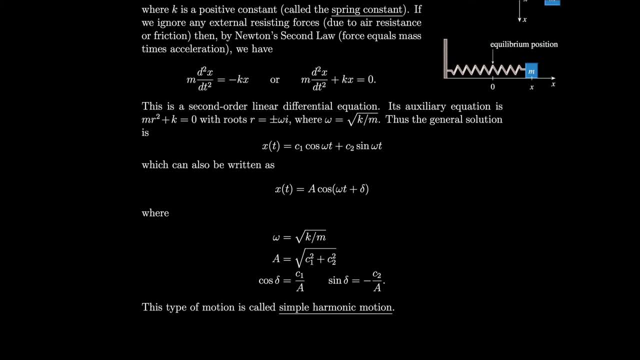 And cosine of delta is c1 over a, but sine of delta is negative- c2 over a- And we call this type of motion a simple harmonic motion. So let's just quickly understand why we can rewrite it. if we were to set this equal to a times cosine of omega t, times c1 over a plus, 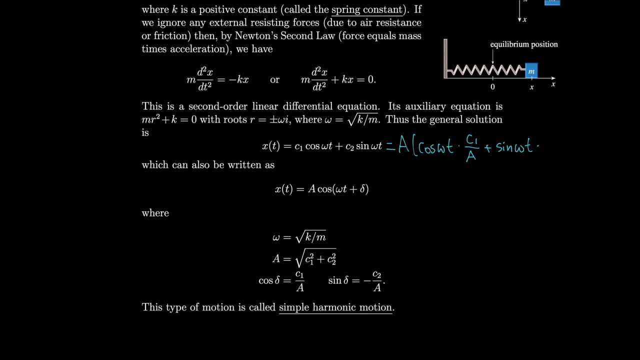 sine of omega t times c2 over a. Then all we've done is multiply on the outside by a and divide on the inside by a. So we just multiply and divide it by the same number. So all we did was multiply by one. We didn't change anything. So what we could then do is write a times the cosine of omega t. 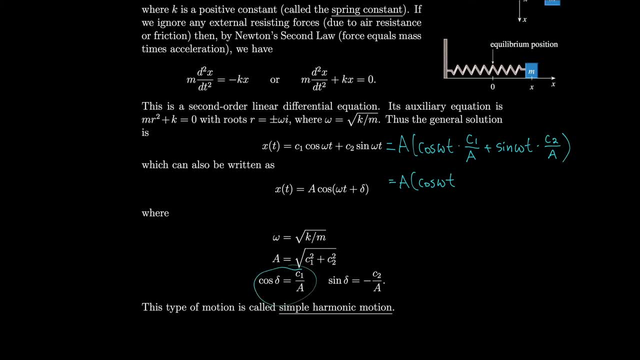 times. well, c1 over a is cosine delta by what we're saying. So this would be cosine delta in here plus sine of omega t times negative sine of delta. So I just put a minus over there. So minus sine omega t times the sine of delta. 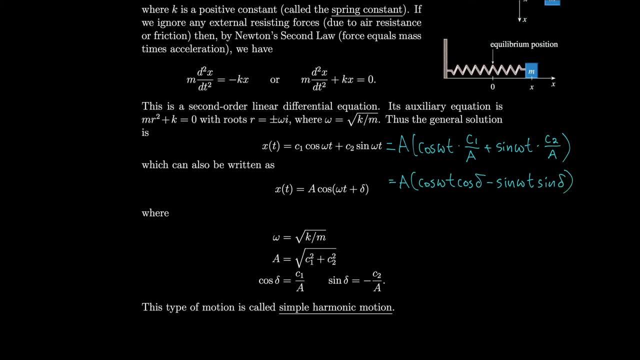 Well, in this case we have cosine, cosine minus, sine sine, two different things: omega t and delta. omega t and delta, So we can use the cosine angle addition formula, And when we do that, we just get cosine of omega t. 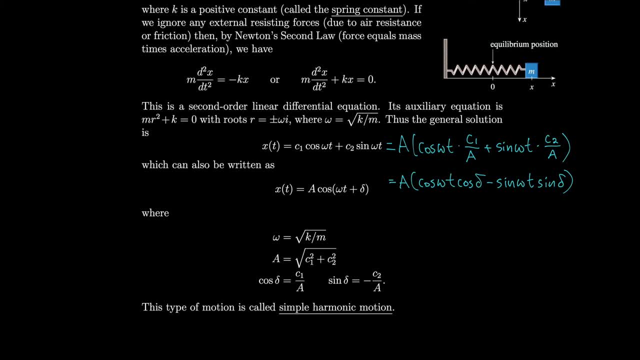 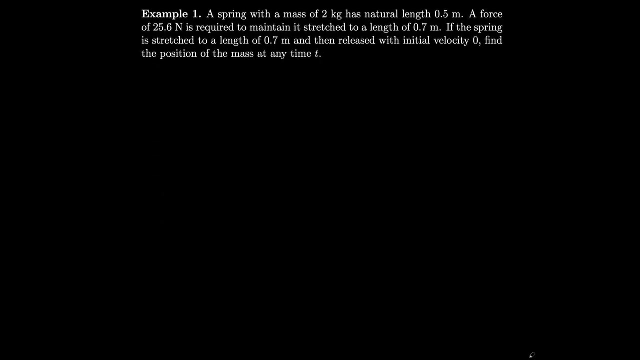 plus delta. So we have a couple of different names for these different things. Omega is the frequency, A is the amplitude, And delta is the phase And delta is the angle. So let's do an example of this: A spring with a mass of two kilograms has natural length 0.5 meters. 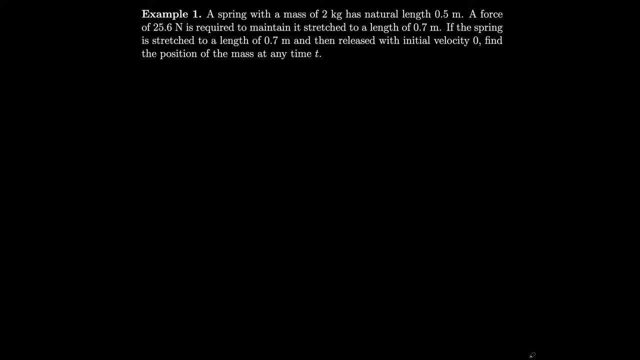 A force of 25.6 Newtons is required to maintain its stretch to a length of 0.7 meters. If the spring is stretched to a length of 0.7 meters and then released with initial velocity zero, Let's find the position of the mass at any time t. 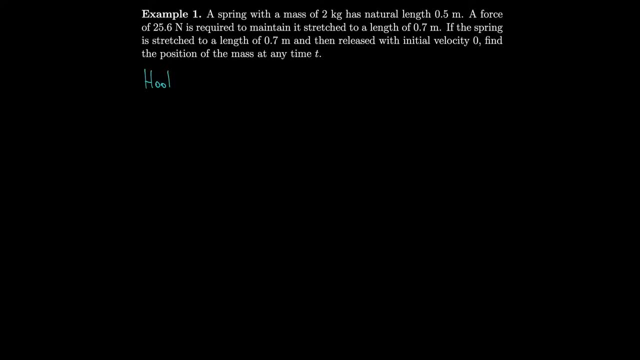 So how about we first use Hooke's law? So according to Hooke's law we have k times how much we've stretched. Let's see we're going from a natural length of 0.5 to a stretch length of 0.7.. 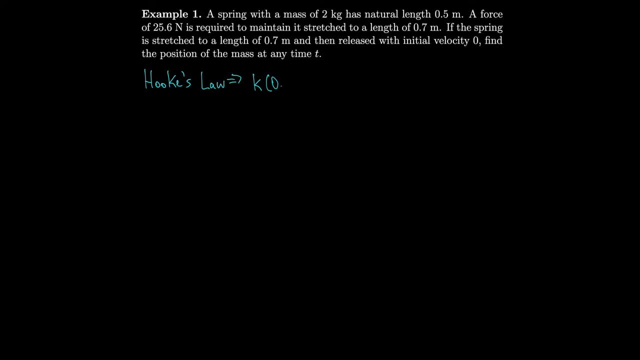 So that means we stretched by 0.2.. So we'll take k times 0.2, and that must equal our force of 25.6 newtons. So that allows us to solve for k. We get that k is equal to 25.6 divided by 0.2, which is 128. 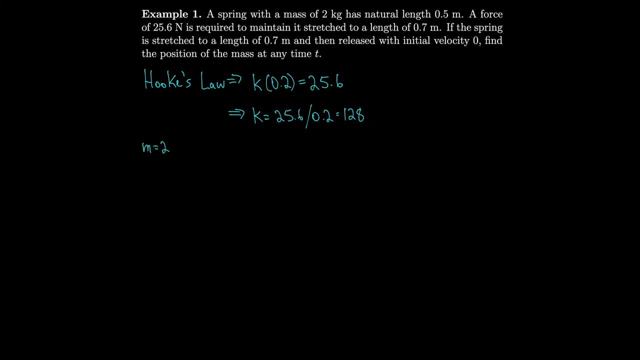 So now we also know that m is equal to 2 because we were told the mass is 2 kilograms. So we can plug that in and get our differential equation. So that's 2 times the second derivative of x with respect to t plus 128x equals 0. 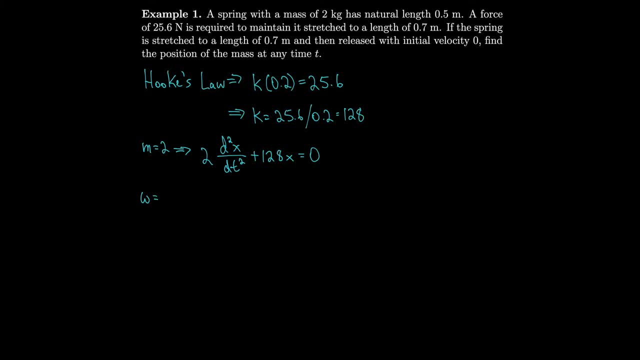 We also have that omega is equal to the square root of k over m, so that's 128 over 2.. So that's 64,, so that's 8.. So that's 8.. The square root of 64. And this means that we can write our solution x of t as c1 times cosine of omega t. 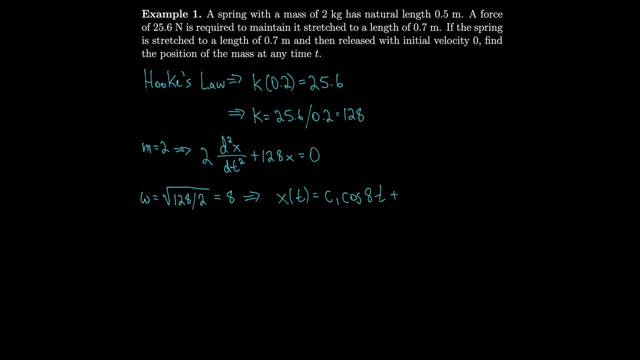 So that would be cosine of 8t plus c2 times the sine of 8t. And we also know that our initial length we are stretched to is 0.7.. So that means we are initially stretched by 0.2.. 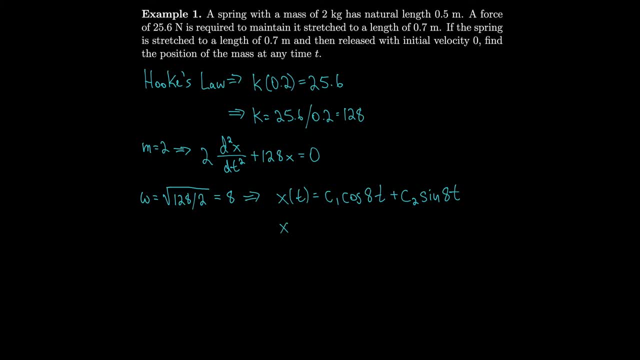 So that means that x of 0, and if we plug in 0 for this, we get this is 0, and this is just going to be c1.. So we get x is 0,, c1, that must be how much we initially stretched by- which is 0.2. 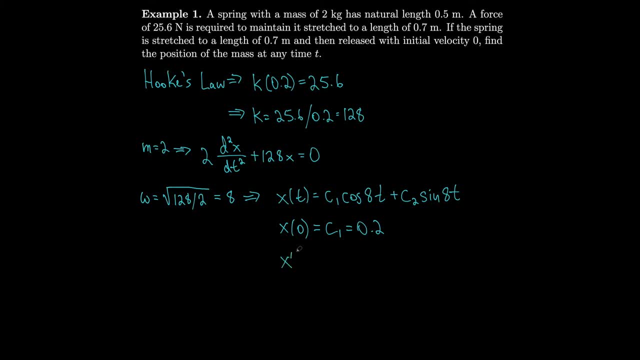 So we know what c1 is. If we want c2, we can take the derivative x prime of t, and that's equal to negative 8 times c1, times the sine of 8t, Plus 8 times c2, times the cosine of 8t. 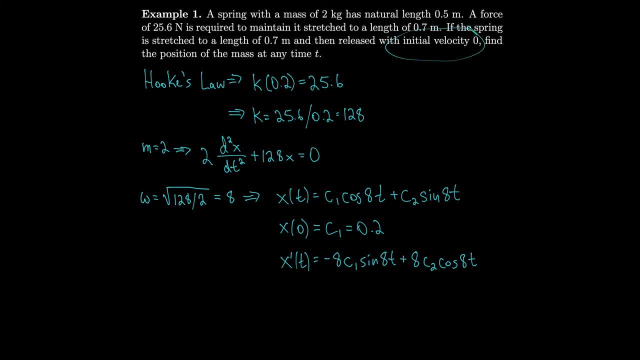 So our initial velocity is 0. So that means that x prime of 0 must be 0. But if we plug in 0 over here, this is 0. We just get 8 times c2 is 0. So that's the same thing as saying that c2 is equal to 0. 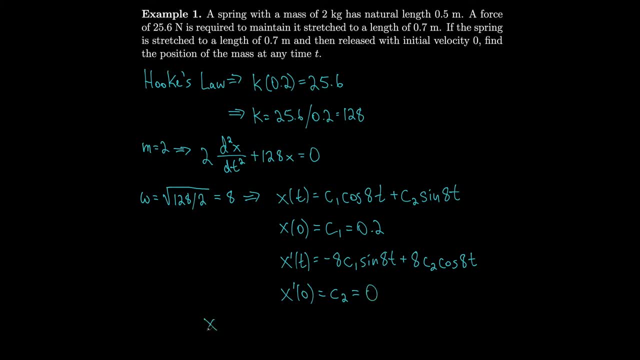 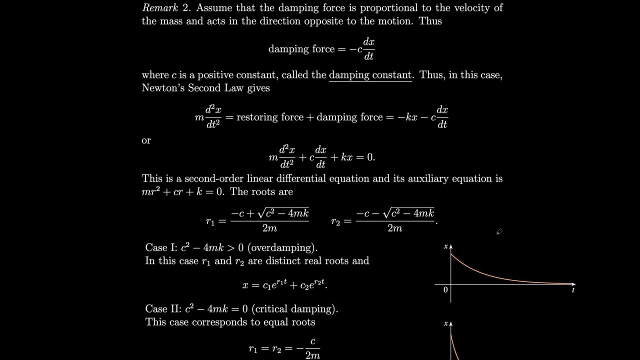 So we have Our position of the mass at the time, t given by x of t equals 0.2 cosine 8t, Because this ended up being 0.. Very often our differential equations in this situation become a little bit more complicated because of external forces such as a damping force. 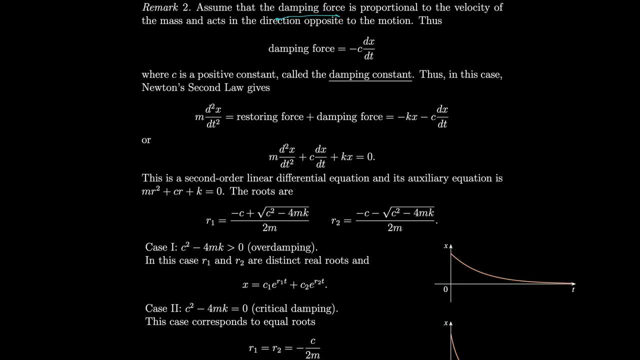 Which is a force like when a spring is submerged in liquid or in reality like a shock absorber on a bicycle. So a damping force affects our differential equation a little bit And we're going to assume that it's proportional to the velocity of the mass in x, in the direction opposite to the motion. 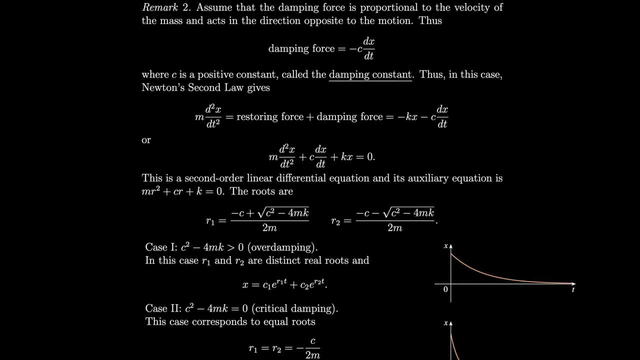 And this can be sort of experimentally determined, but of course we're not going to do that. So we have our damping force equal to negative c times dx Or c is a positive constant called the damping constant. So then Newton's second law gives m times the second derivative of x with respect to t. 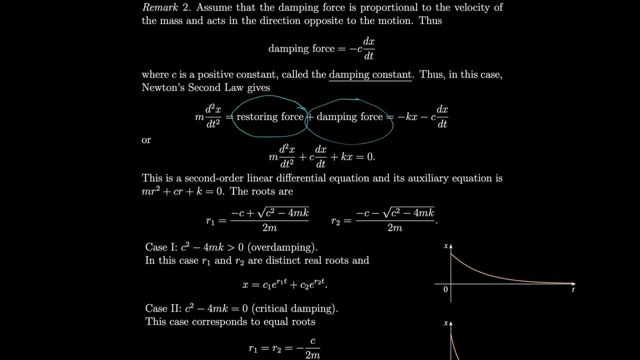 equal to the restoring force plus the damping force. So that's negative kx plus negative c times dx, dt. So that means that when we move everything over to one side and set it equal to 0, we end up with still a homogenous differential equation. 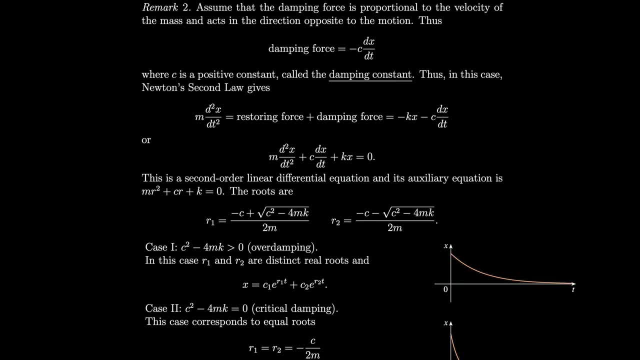 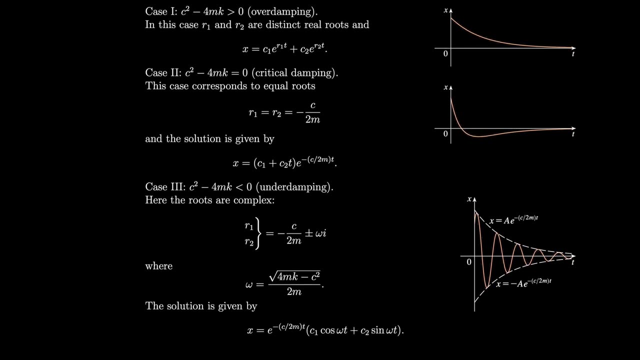 But it's slightly more complicated. So now it has auxiliary equation: m, r squared plus c, r plus k equals 0. So its roots become a little bit more complicated using the quadratic formula. So we end up with a couple different cases. Our first case is that if we have the discriminant c squared minus 4mk, greater than 0,. 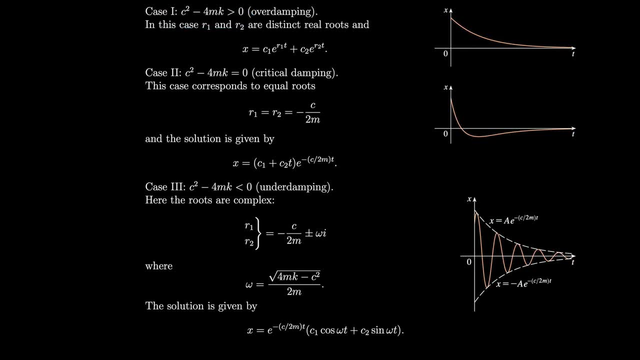 then we have overdamping. So in this case we have r1 and r2 as distinct real roots. So our solution to our differential equation is given, as we would expect, with c1,, c2, and c3. So we have e to each of those roots, c2, e to the other root. 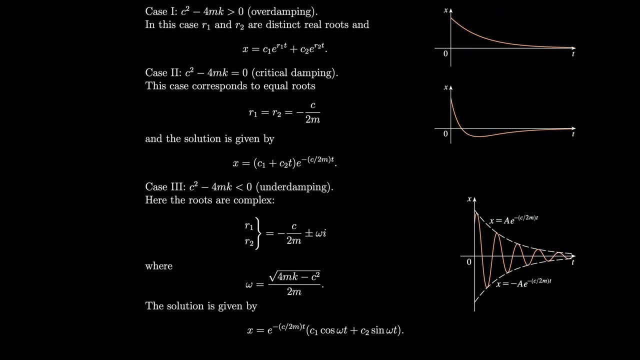 And it looks something like this in this picture, where the shock absorber you can imagine- or damping force, whatever you want to think of it- as is preventing this thing from oscillating. It can only really cross the axis one time. 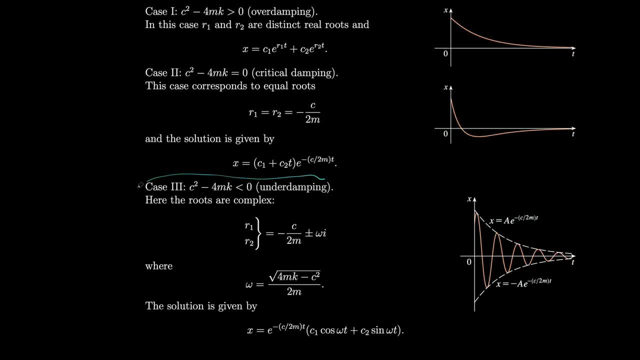 Whereas if we have underdamping, then we have the discriminant negative. And we have the discriminant negative And notice it oscillates tons because we didn't dampen enough, So we didn't absorb the shock. So in that case we have roots given by complex numbers. 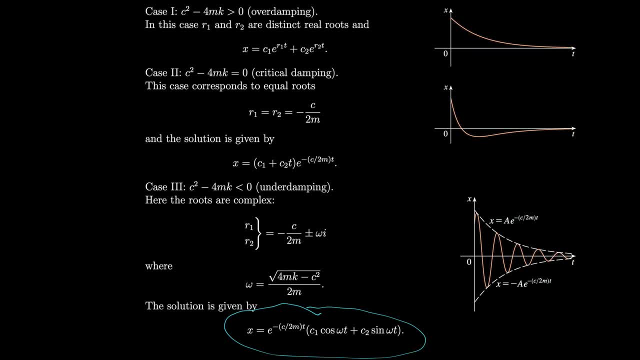 And our solution is given, as we would expect, e to the alpha t times c1 cosine beta t plus c2 sine beta t, where alpha is negative, c over 2m and beta is omega. So we end up with a solution to our differential equation. 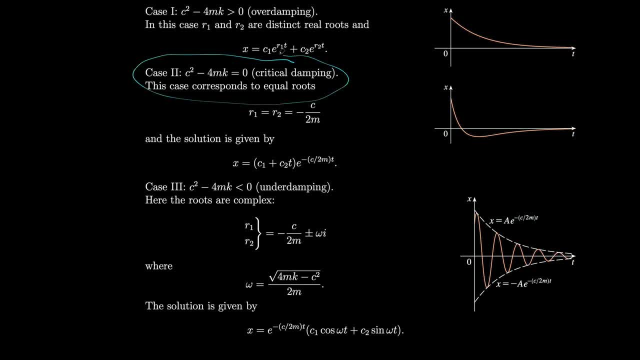 So we end up with a solution to our differential equation. But the last case, where- well, the middle case, however you want to think about it, where we have critical damping, is pretty similar to overdamping, We just end up with one real root. 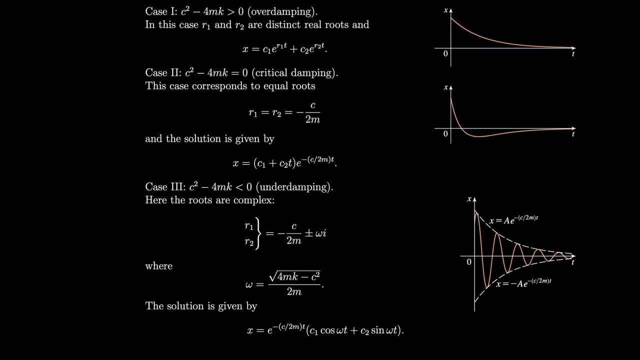 We throw in a t like we threw in x And we get our solution. And it looks similar to when we had overdamping. So this is basically just when you damp like exactly enough, You absorb exactly enough shock. think of it as: 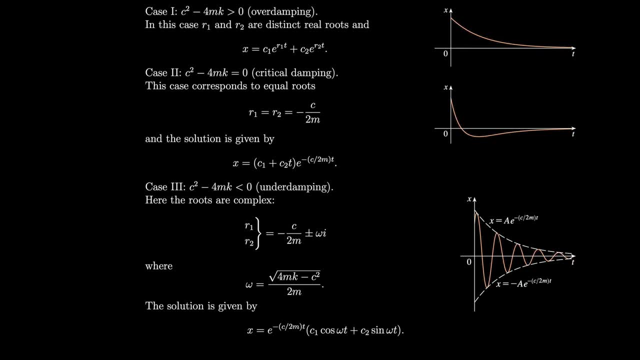